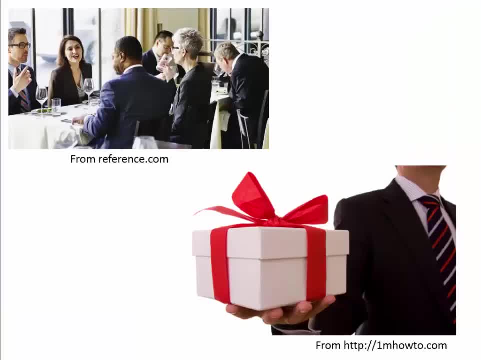 it had higher gas mileage. The use of this defeat device is an obvious ethical violation. Most ethical issues will not be this obvious Ethical questions can arise when accepting gifts or meals from contractors, accepting outside employment or when comparing non-disclosure agreements to the public's right to know certain information. Fortunately, there are codes of. 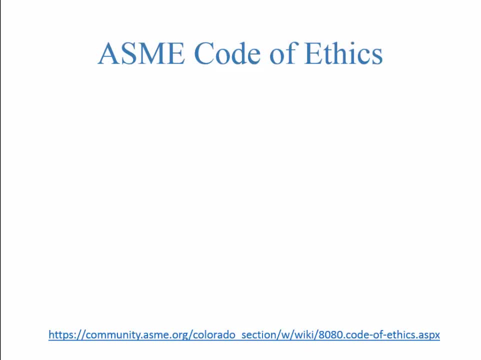 ethics that have been developed to help guide young engineers in their ethical decision-making. Many professional organizations publish their own code of ethics, including the American Society of Mechanical Engineering. This code has three prerequisites: Primary principles, which state that engineers uphold and advance the integrity, honor and 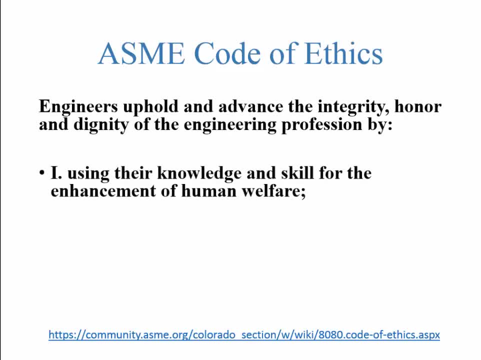 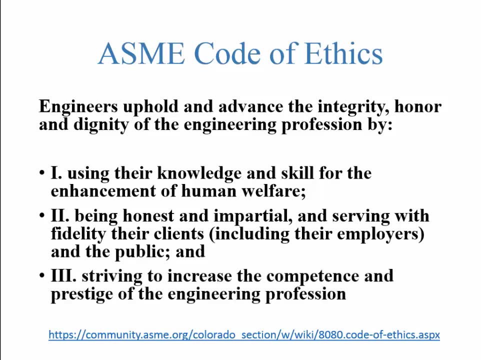 dignity of the engineering profession by: one, using their knowledge and skill for the enhancement of human welfare. two, being honest and impartial and serving with fidelity their clients, including their employers, and the public. and three, striving to increase the competence and prestige. 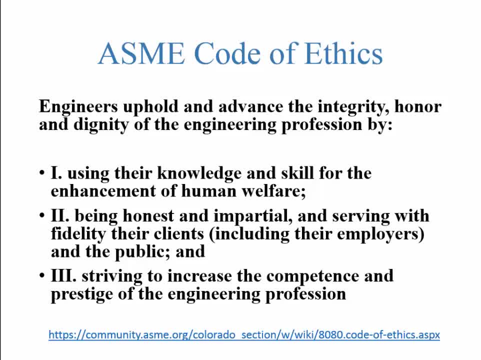 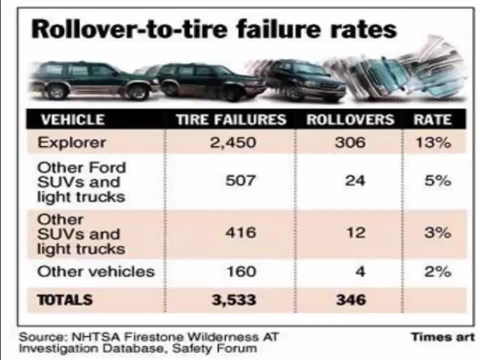 of the engineering profession. There are also eight canons that help explain these principles, and further clarification can be found at the website shown. Another famous case study involves a Ford Explorer and Firestone Wilderness AT tire In the late 90s. it was noticed that there was a much higher rate of tire failures and rollover. 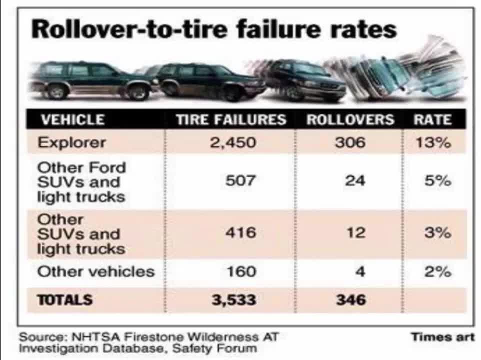 rates on Ford Explorers equipped with the Firestone Wilderness AT tire. Although there is some evidence that both companies knew about these failures, nothing was done until 2000, when NHTSA began an investigation. The two companies blamed one another during numerous lawsuits. 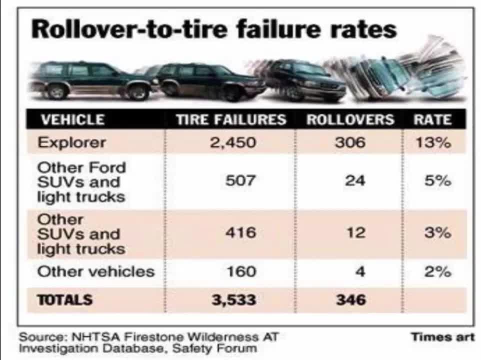 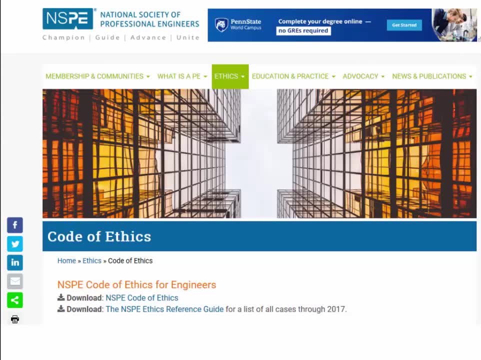 and the companies ended up severing a relationship that had lasted over a hundred years. To help guide engineers through potential ethical conundrums, the National Society of Professional Engineers has also established a code of ethics, Similarly to the ASME code. it contains some 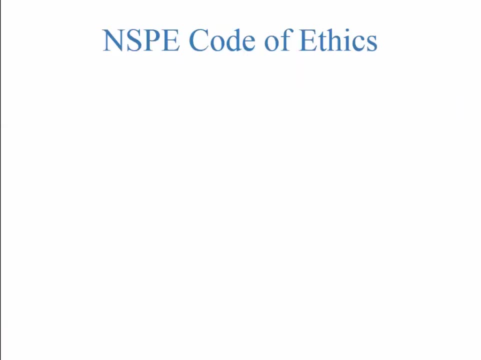 fundamental canons as well as additional guidance. Their fundamental canons state that engineers, in the fulfillment of their professional duties, shall hold paramount the safety, health and welfare of their employees. The code of ethics is a code of ethics that is used to establish a 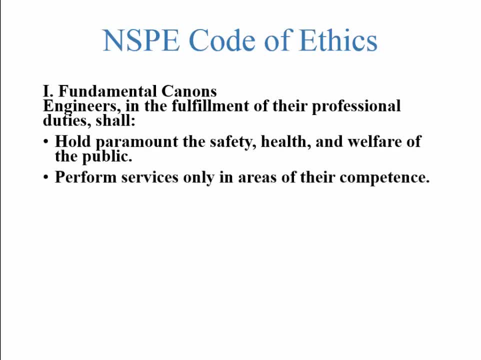 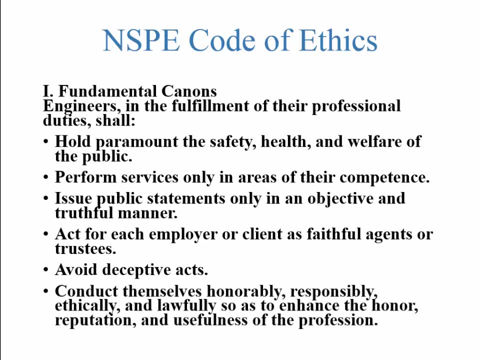 rule of the public. perform services only in areas of their competence, issue public statements only in an objective and truthful manner. act for each employer or client as faithful agents or trustees, avoid deceptive acts and conduct themselves honorably, responsibly, ethically and lawfully, so as to enhance the honor, reputation and usefulness of the profession. 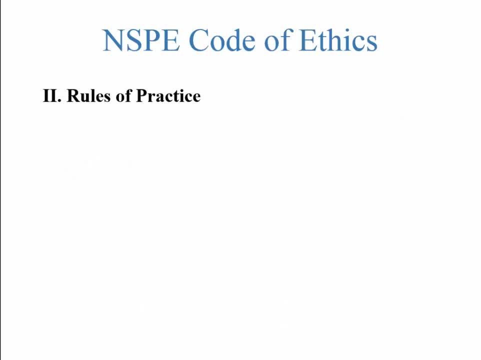 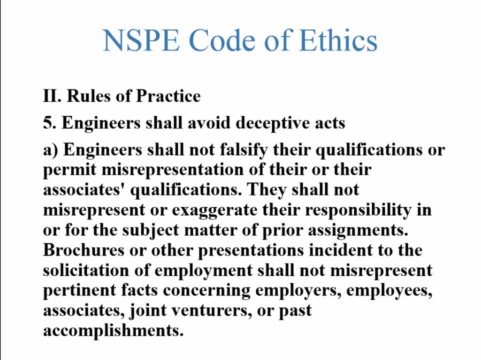 It also has a set of rules of practice. For instance, under engineer's rules of practice, the code of ethics says that engineers- engineers- shall not falsify their qualifications or permit misrepresentation of their or their associates' qualifications. They shall not misrepresent or exaggerate their responsibility. 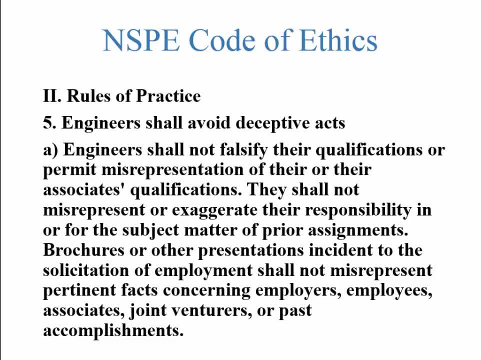 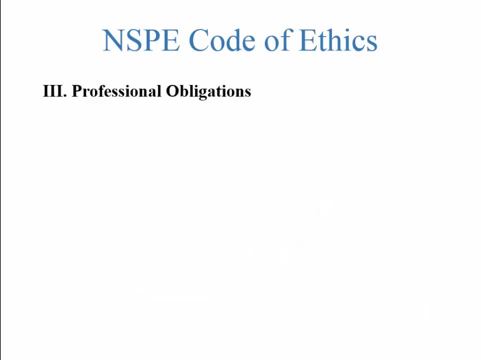 in or for the subject matter of prior assignments. Brochures or other presentations incident to the solicitation of employment shall not misrepresent pertinent facts concerning employers, employees, associates, joint ventures or past accomplishments. There's also a list of professional obligations. They discuss things that engineers should do, Things like act with. 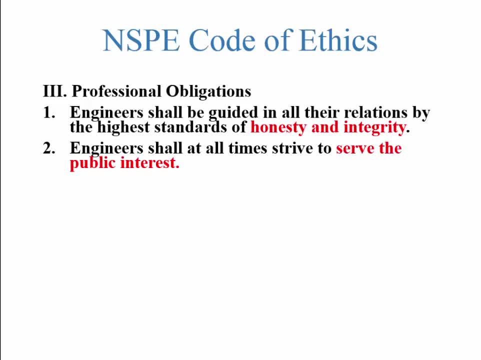 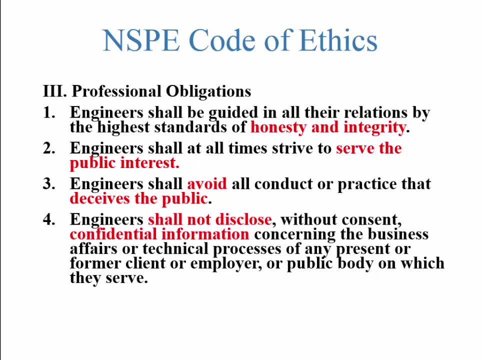 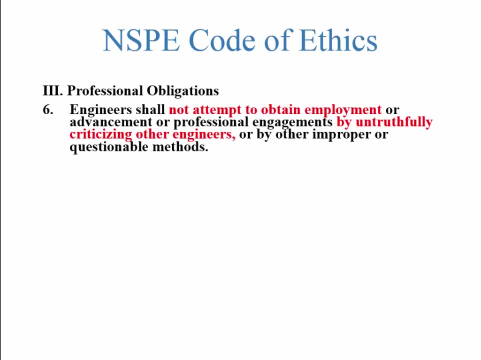 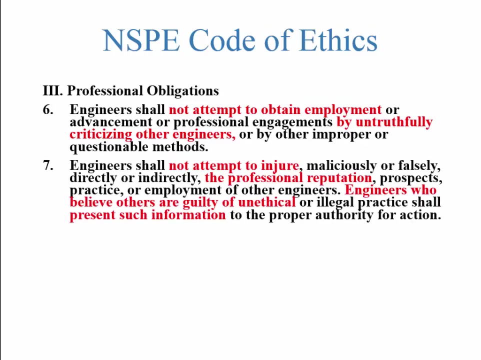 honesty and integrity serve the public interest. avoid deceiving the public, such as in the Ford, Firestone and VW cases. not disclose confidential information and avoid conflicts of interest. Additional obligations are not to obtain employment by criticizing other engineers, don't injure the professional reputation of other engineers and that you should turn in those. 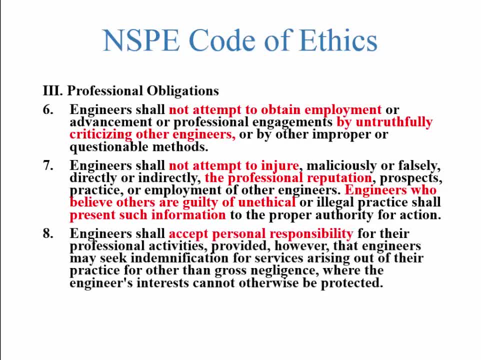 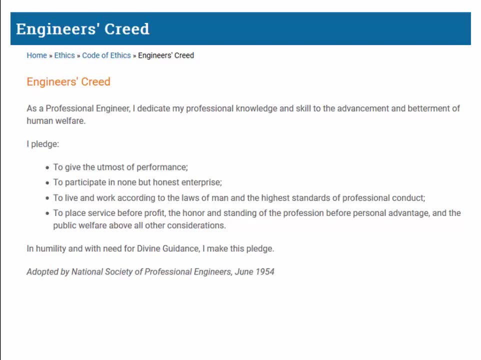 who act unethically. Finally, you should accept personal responsibility for your activities and you should give credit to others where credit is due. There's also an engineer's creed that says: as a professional engineer, I dedicate my professional knowledge and skill to the advancement and betterment of human welfare that I pledge to. 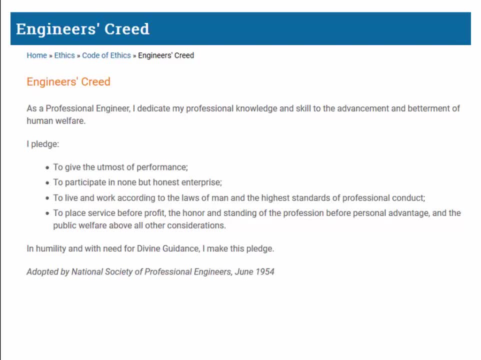 give the utmost of performance, to participate in none but honest enterprise, to live and work according to the laws of man and the highest standards of professional conduct, and to place service before profit, the honor and standing of the profession before personal advantage and the public welfare above all other considerations. 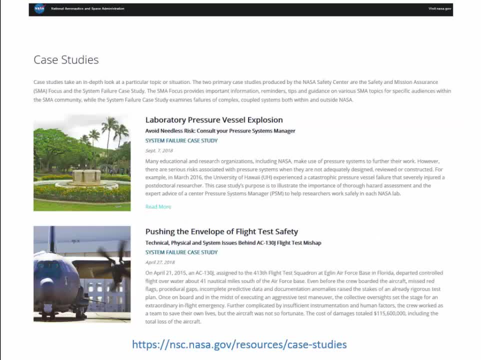 NASA maintains an interesting website containing recent case studies where ethical issues may have arisen. We encourage you to look through these case studies so you can see other instances where ethical issues have occurred in engineering practice.